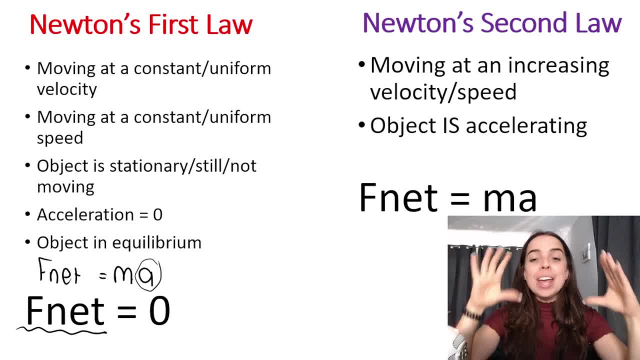 is zero, f net is equal to zero, So f? net is equal to zero is how we basically start off our Newton's first law calculations. If you've missed the video where I go through how to use your free body diagram to help you set up force equations, you may want to check that out, because that's. 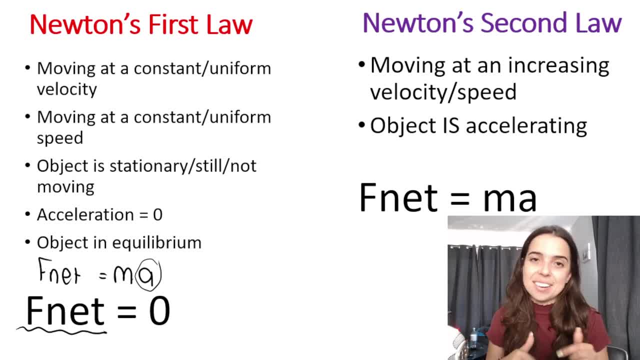 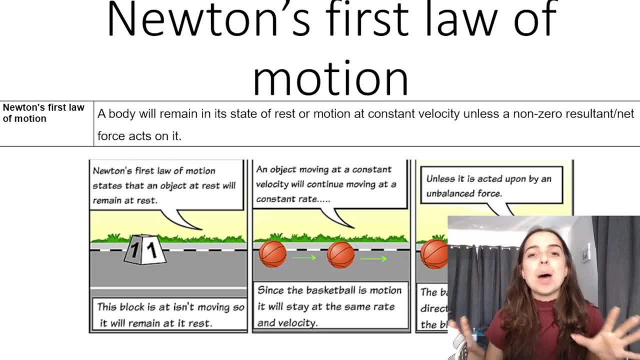 going to be very helpful for both Newton's first law and second law. I'll link that in the description box below. but it's very important to first make sure you are doing the correct type of math. But hold up before we get to a calculation. what is Newton's first law of motion? So you can. 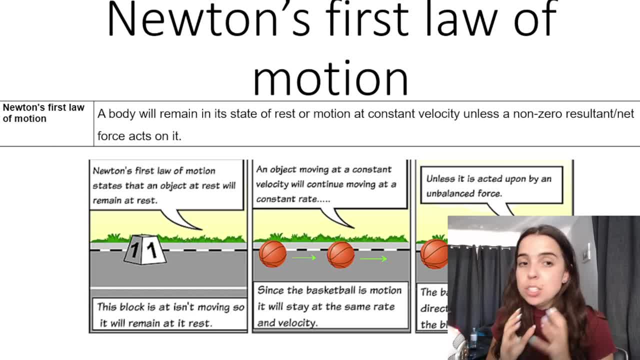 see the definition at the top of the screen behind me. So it says Newton's first law of motion: a body will remain in its state of rest or motion at a constant velocity unless a non-zero resultant or net force acts on it. So you can see in the definition that they mention both a state of 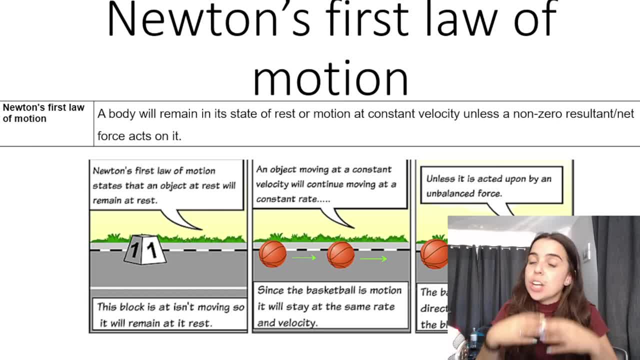 rest, so staying stationary or still, or motion at a constant velocity, Constant speed, constant velocity, uniform velocity. So they say, if those are the cases, then we are dealing with Newton's first law of motion and a body will stay in the state of motion or state. 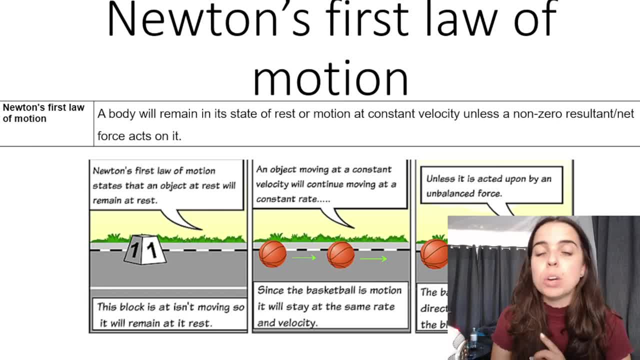 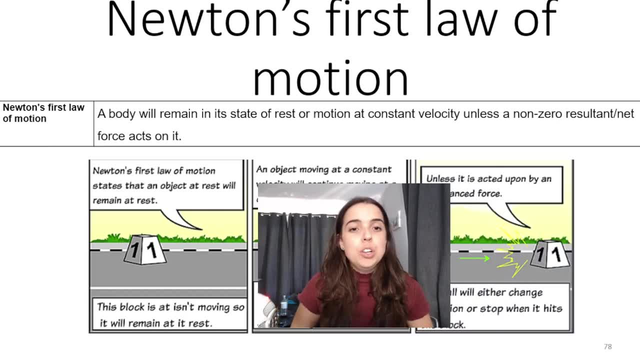 of rest unless a non-zero resultant or net force acts on it. Now what does this mean? If you take a look at these pictures behind me, the first picture says: Newton's first law states that an object will remain at rest. So you can see that that cone over there in this picture, the block, is not moving. 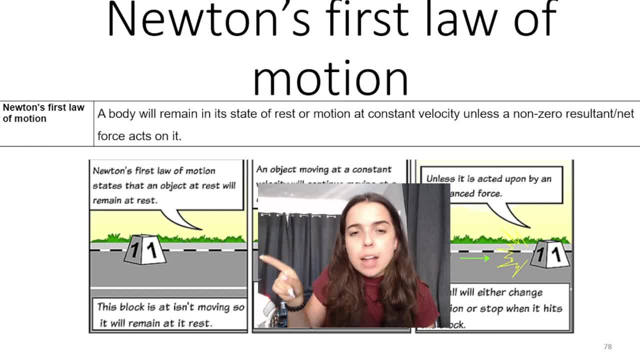 So that block will stay still. Until when will that block stay still? And you could say, well, ma'am, someone could come and push it over, and then it'll move. and you are right, It will move in that scenario because a non-zero net force or resultant force is acting on it, a pushing force, which is a. 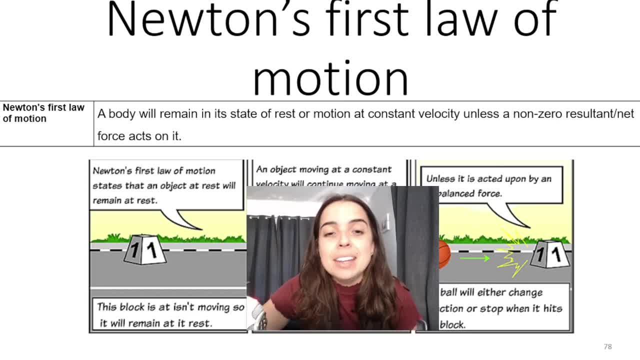 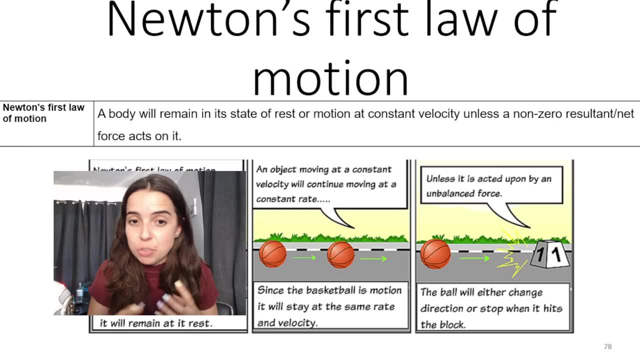 net force, a non-zero net force, And in the same way we can see this picture over here. so it says an object moving at a constant velocity will continue moving at that same velocity or speed. So if the basketball is in motion, it will stay in motion and technically, if the surface is, 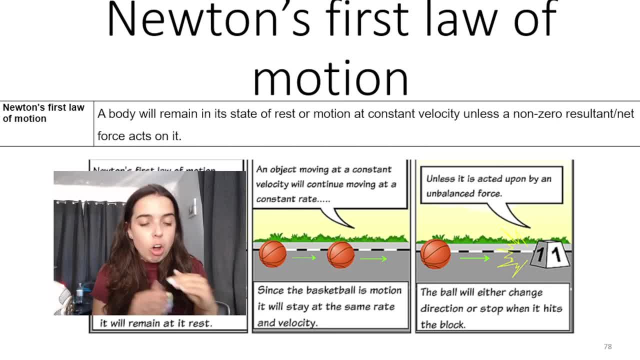 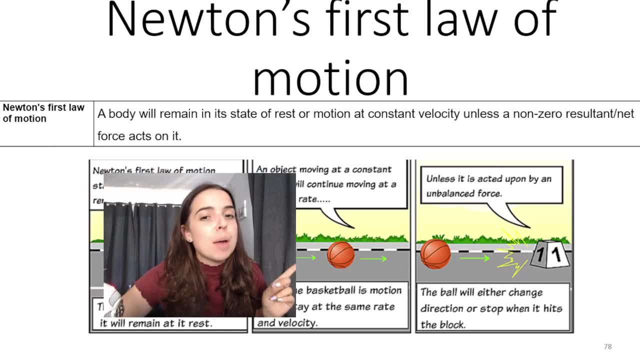 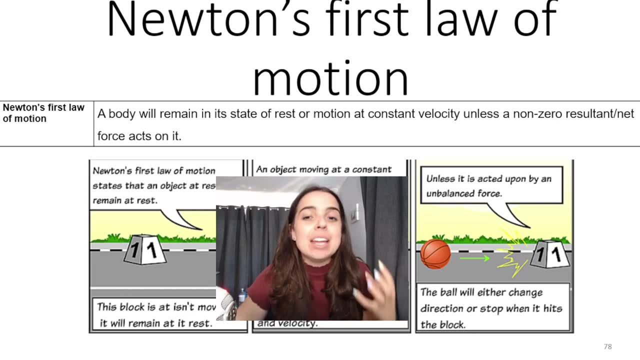 frictionless, it will stay in motion forever. So if I kick a ball on a truly frictionless surface, it will carry on like that forever. according to Newton's first law In this sequence of diagrams it doesn't continue forever. Why? Because look at the ball. it hits the cone and what happens is a. 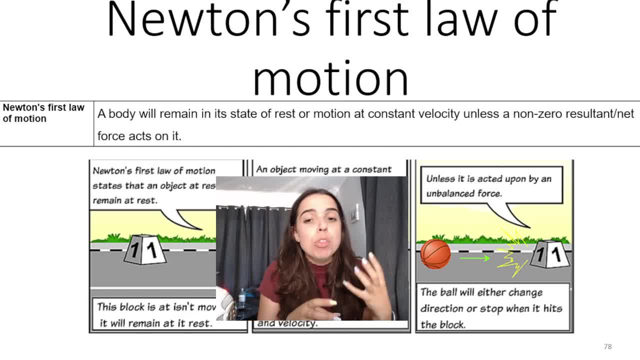 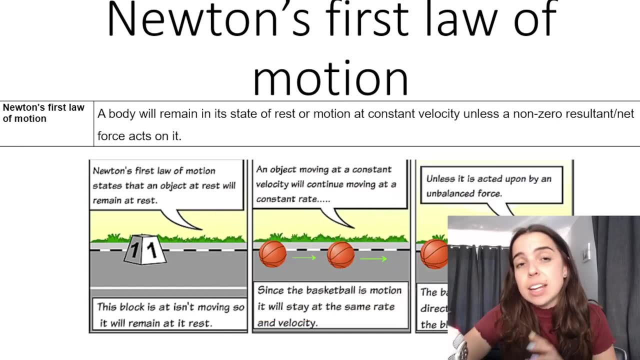 non-zero net force is acting on the ball, Which is causing the ball either to stop, slow down, change direction, in other words, causing the ball to accelerate. Okay, so that is Newton's first law: An object or body will remain in its state of motion or rest at a constant velocity if it's in that motion, unless a non-zero resultant or net. 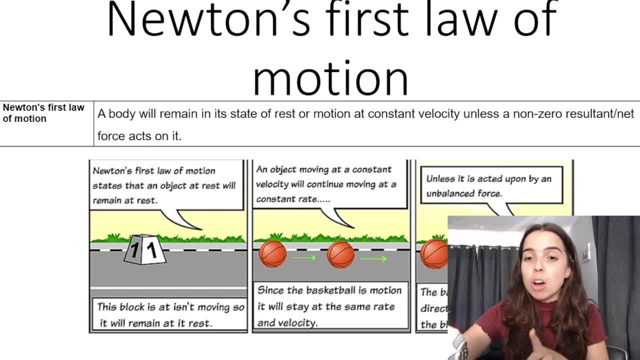 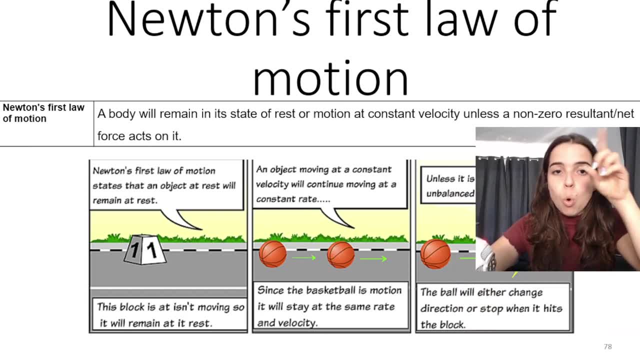 force acts on it. Now, teacher tip: I set metric papers, I mark them. so I know that if you don't say non-zero, they take away a mark. If you don't say resultant or net, you can choose, they take away a mark. You need to say these things. 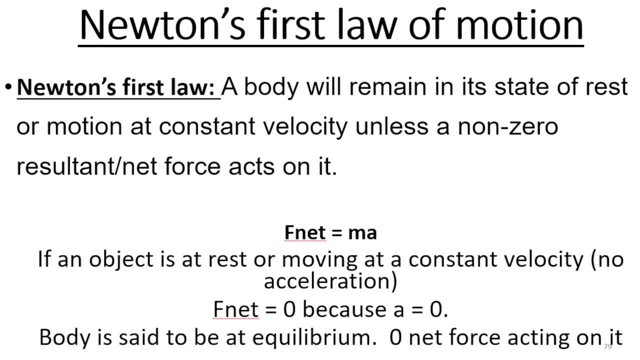 in order for you to get your full marks for your definition. So here's a repetition of the definition for you. This definition comes from your exam guidelines, so this is the correct definition. You will see alternative definitions on the internet, in weird textbooks, weird videos on the. 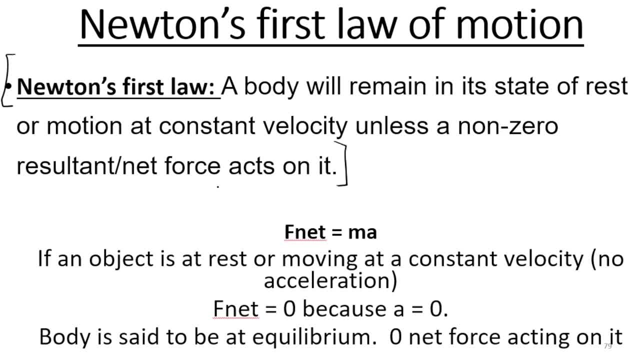 internet. but this is the correct definition according to your exam guidelines. Okay, cool, F net equals ma. Remember we technically should start all Newton's law questions like this Newton's first and second law, but remember I did tell you that F net equals zero if we're dealing with a Newton's first law. 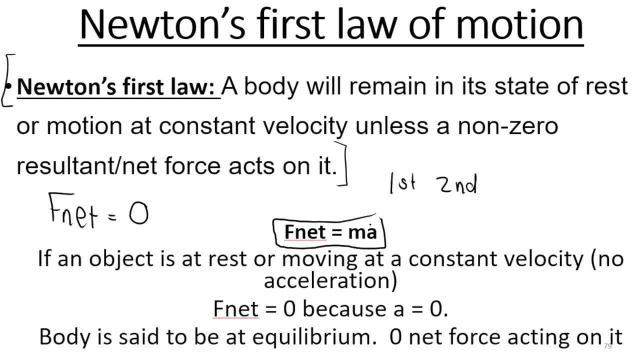 question. and the reason why F net equals zero, ultimately, is because acceleration is zero. because, remember, the object is either not moving, which means acceleration is zero, or it's moving at a constant velocity, which means acceleration is zero, So the body's in equilibrium, there's zero. 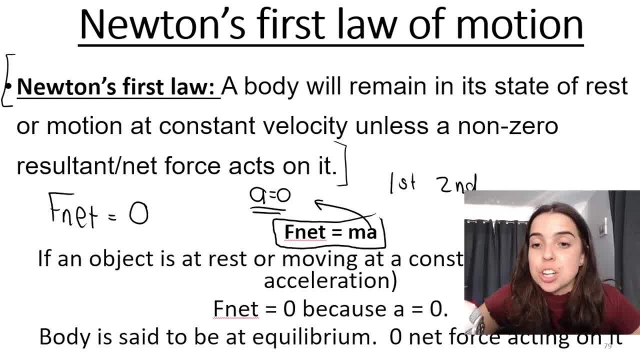 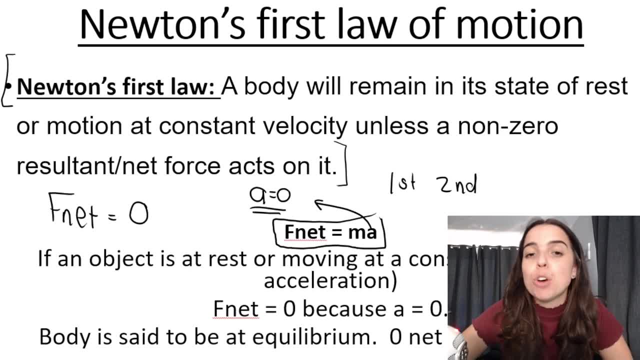 net force acting on it. Now, before I go into a calculation, there is something very important that you need to know. according to exam guidelines, you do need to know safety considerations in terms of Newton's first law of motion. So you could be like ma, what are you talking about? You need to understand why it. 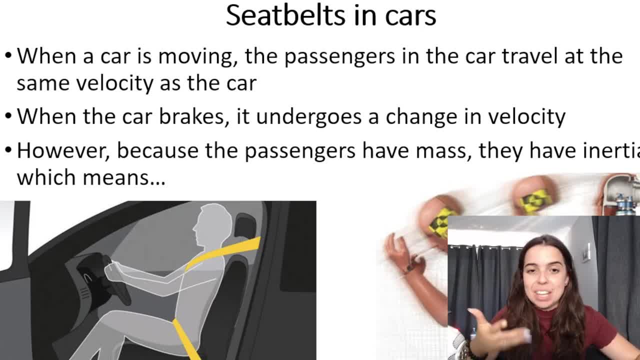 is important for us to wear seat belts when traveling in a car. Now think about this: you're sitting in a car. you do not have your seat belt on. okay, you're sitting in a car, the car is going at 120 kilometers per hour. that's very fast, very, very fast. So you need to know safety considerations. 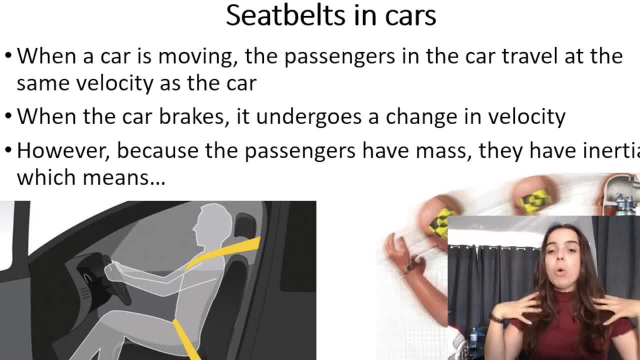 you because you're in the car, you are traveling at the same constant velocity: 120 kilometers an hour. now, what happens if the car breaks? what happens? so think about it. if the car breaks, okay, it's negative acceleration, the car is slowing down, it's changing its velocity. however, the passengers 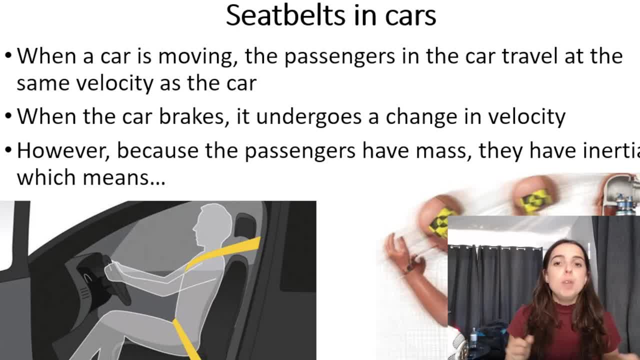 so, in this case, me- I'm pretending to be a passenger in a car because I have something called inertia, Because I have mass. that means that I do want. I want to resist any change in motion. so because I have mass, I have inertia, which is just a property of a body: it resists change in motion. so because 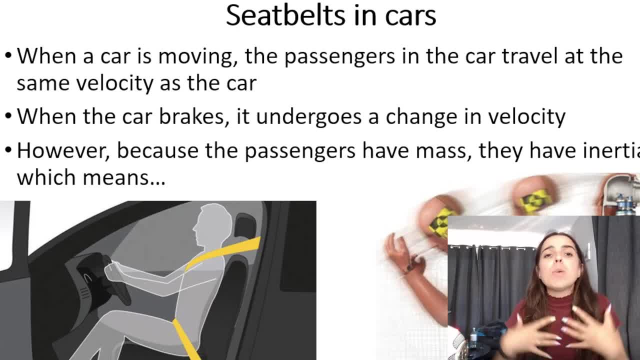 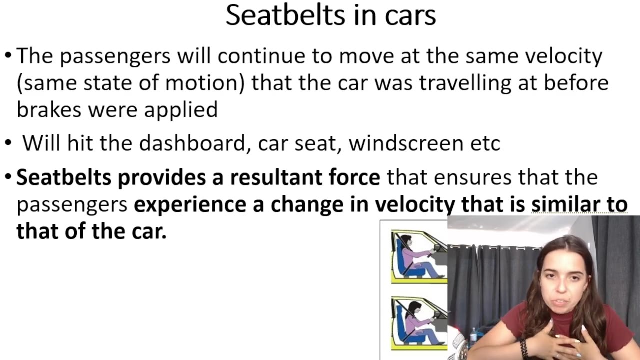 I'm traveling at 120 kilometers per hour. I want to continue traveling at 120 kilometers per hour. this is also according to Newton's first law. Newton's first law says: I'm at motion at 120 kilometers an hour- constant velocity. I will continue to do so at the same velocity that the car. 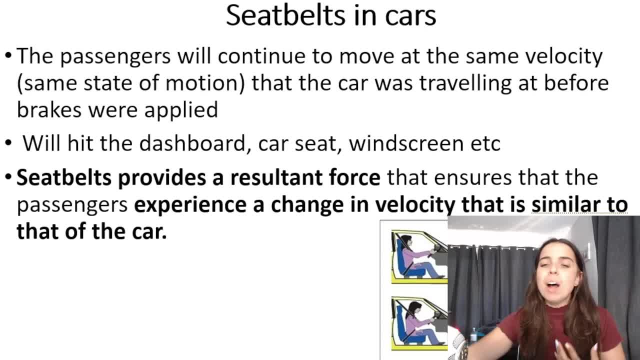 was moving at. my body wants to continue traveling at the same constant speed. So when the car breaks, I will continue to move at the same velocity that the car was moving out before the brakes were applied and I will fall forward. I will fly forward. it's not a good thing for me. 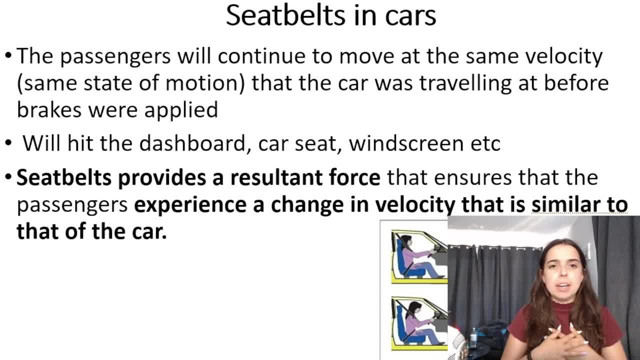 What does wearing a seat belt help with? Well, the seatbelt provides the nonzero result and force and it's a backwards for. so think about if you've ever been in a car and you've been wearing a seatbelt and the car suddenly got a bit on your hands and it suddenly reaches like this: 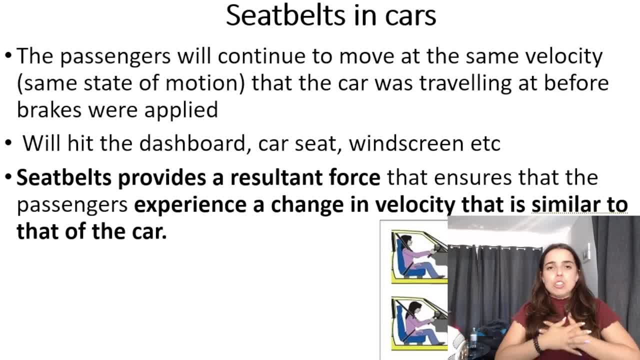 and the car suddenly comes to a stop, that seatbelt pulls you back quite sharply against your seat. So the seatbelt provides a resultant, a non-zero resultant or net force, and it basically ensures that my velocity changes in the same way of the car. So when the car slows down, I slow down. 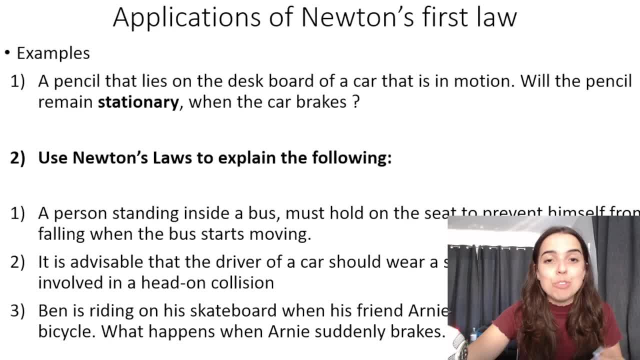 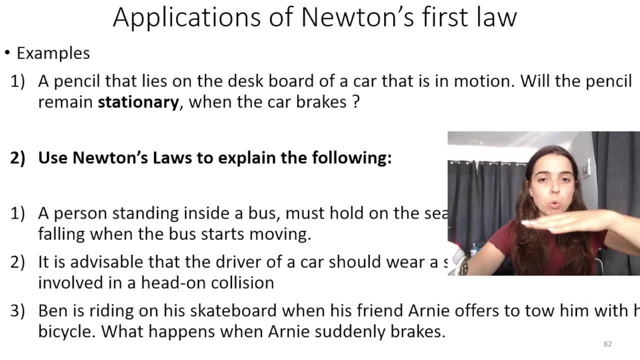 So you need to be able to use Newton's first law, apply Newton's first law to explain these various scenarios. So, for example, if a pencil lies on a dashboard or a dashboard of a car that is in motion, will the pencil remain stationary when the car breaks, Unless there's something holding? 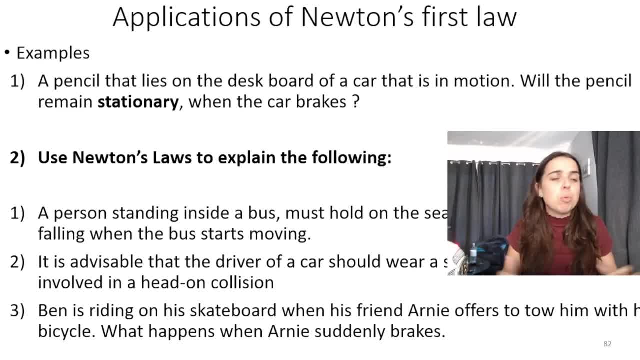 onto the pencil. the pencil won't remain stationary. It will want to continue at the same constant velocity, according to Newton's first law. so it'll stay in that state of motion, at that same velocity. So when the car's velocity decreases, the pencil's velocity won't. It'll continue at the 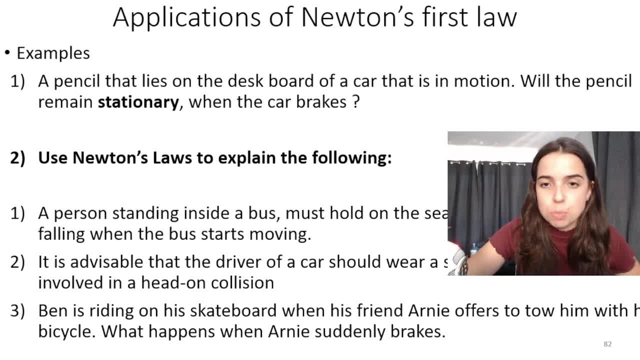 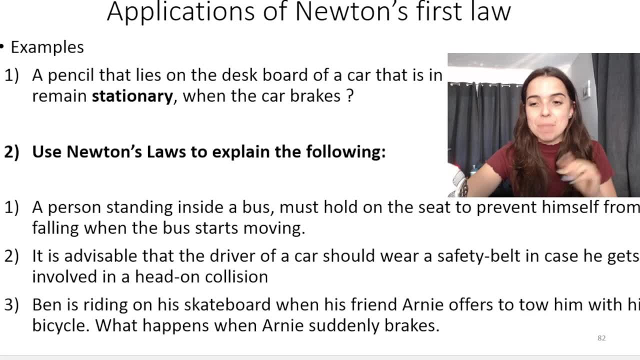 same velocity and it'll fall off the dashboard, Or roll off the dashboard, And you can use that same argument for all of these scenarios over here. Okay, now that we know the theory, let's jump into a Newton's first law: calculation. 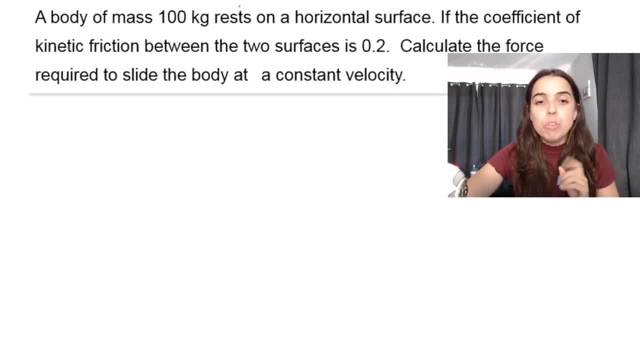 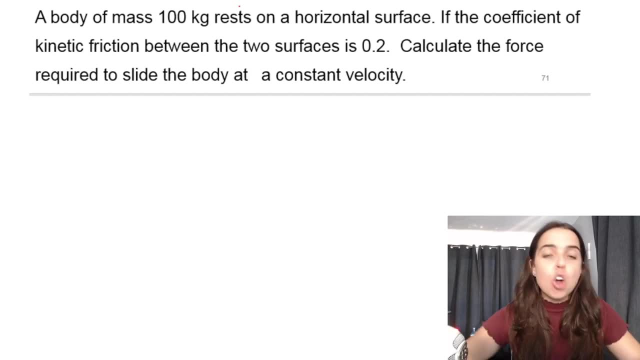 So this is an example of a Newton's first law question. We've got a body, so a box or whatever, or a person or whatever, of mass, 100 kilograms. let's say it's a box rests on a horizontal. 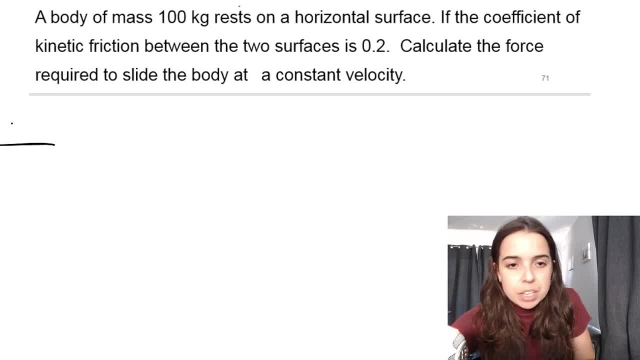 surface. So they don't give me a picture, I'm just going to draw you a picture. Here's my box, it's 100 kilograms, it's resting on the surface and they give me the coefficient of kinetic friction. so that is this little symbol over here, is 0.2, my mass is 100 kilograms. and look what? 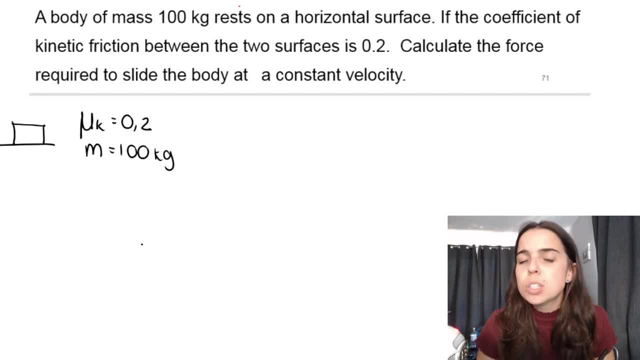 the question wants Calculate the force required to slide the body at a constant velocity. Now, the reason we know it's a Newton's first law question is because of the wording constant velocity. that means that acceleration is zero and therefore, remember, f net is equal to. 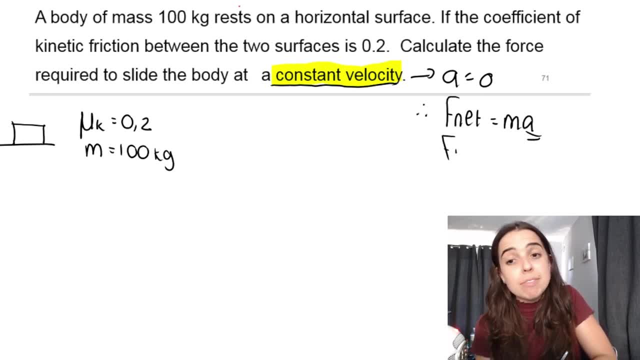 ma. but if a is zero, f net is zero, and we know it's a Newton's first law question. Now, I find questions like this very, very difficult to do, especially as they get more complicated, unless I have a free body diagram. They didn't ask me to draw one, but I'm going to draw one because it 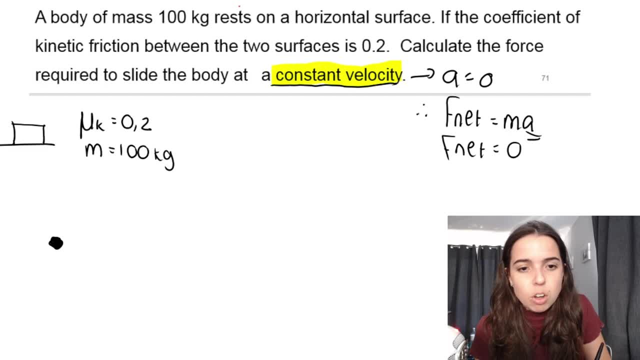 helps me so much with my question. So a box resting on a flat horizontal surface sits on a flat horizontal surface. we know we're going to have a normal force acting straight up, that's Fn because there's a surface involved. We know we have Fg acting straight. 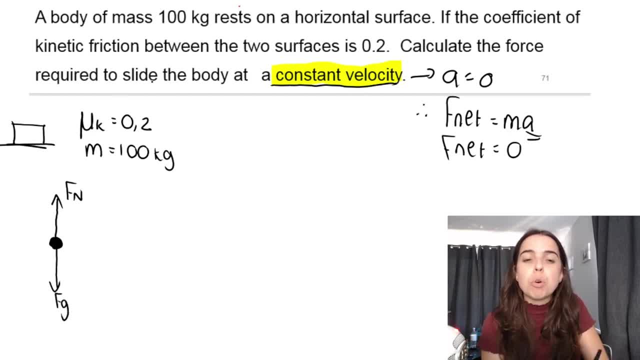 down. They say they want me to calculate the force required to slide the body at a constant velocity. So obviously we're going to have an applied force acting in one direction. so let's pretend it's going to the right. That's F applied, that's the force required to slide the box. 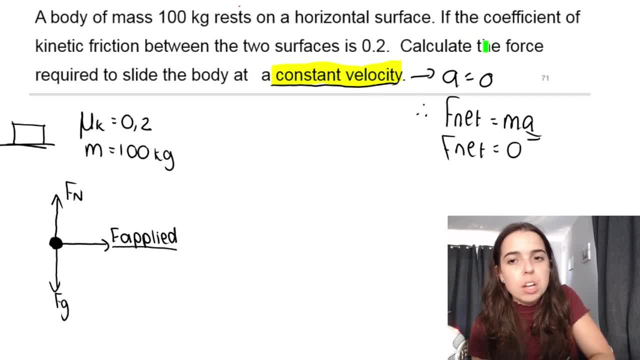 I'm going to highlight that, just so we can see. that is what I'm actually looking for: Calculate the force required to slide the body. I'm looking for F applied. cool, Now they do say that there's a coefficient of kinetic friction. 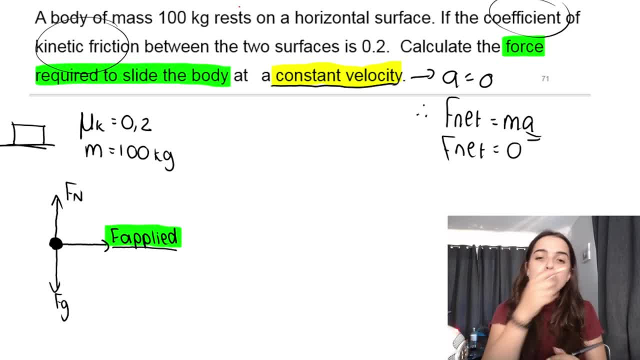 Say Fk from the surface, Let's say so. Let's say Fk for rons, Let's say for advocating the force that's going to act in one direction, and say Fk forу walls, which means that there's obviously friction present And if the box moves to the right friction, 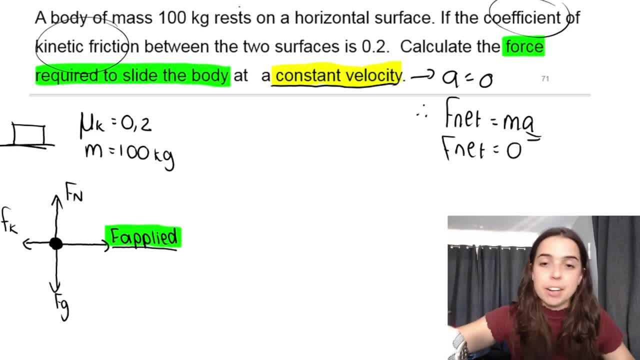 goes to the left and is parallel to the surface. So I'm going to say Fk for kinetic friction. Now you have to always assume that there's friction present, unless they say frictionless, L perseverance friction. we have to assume that there's kinetic friction unless they say that the surface friction. 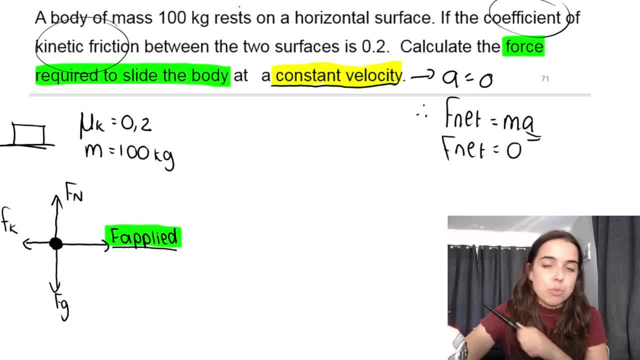 lists. remember, if you don't understand any of these individual forces, i have videos on all the individual forces, also how to draw free body diagrams, so that's linked down below. but drawing it is very important because it helps me understand and answer the question. i think at least so again. 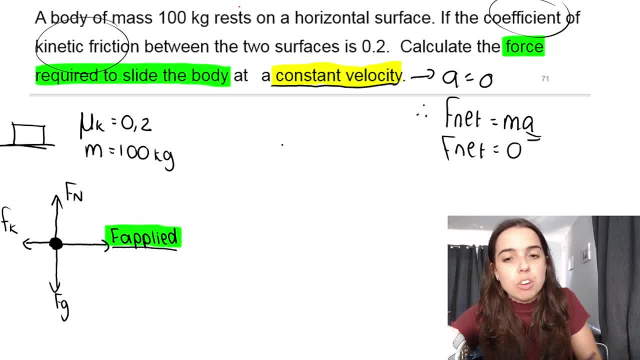 we know it's a first law question. so we know f net is equal to zero. so i'm going to write: f net is equal to zero. they want us to calculate the force required to slide the body or to move the body to the right at a constant velocity. so i'm looking for f applied now in my one video where i mentioned: 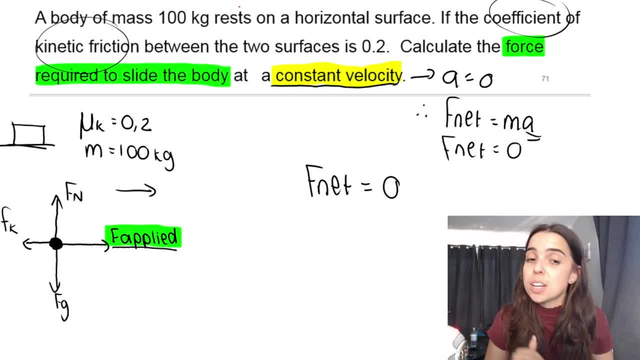 the equations for newton's laws, and i said you must watch this in order to understand newton's laws. i said that if we're looking for f applied, or if we're looking for any force in the horizontal direction, so the parallel direction or the x direction. so in this case i'm looking for f. 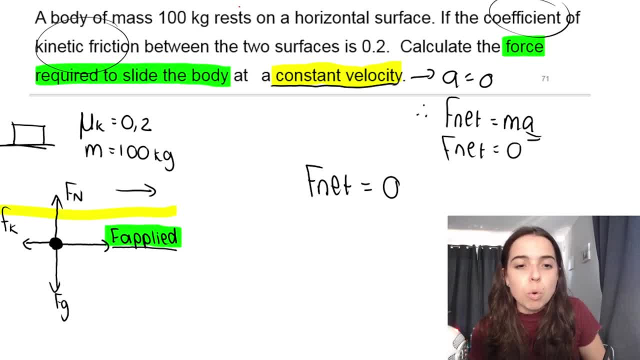 applied, which is in that direction. i need to calculate the force required to slide the body or to move the body to the right at a constant, all the forces in that direction, which would be both of these forces, f applied plus fk. both of those forces i need to consider. and you might say why, ma'am? because remember the 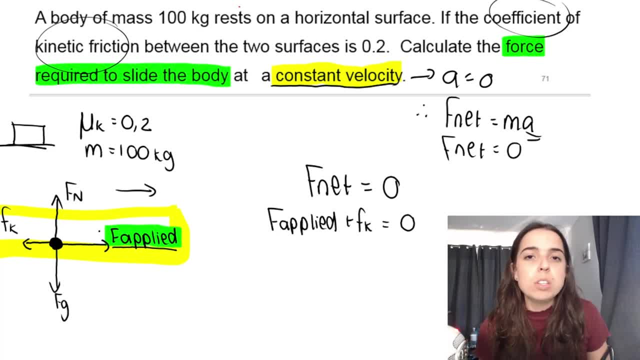 box is sliding in the horizontal direction, so the two forces that affect that motion would be f applied and fk. that's why i need to consider both of them. i need to add them together. when i add them together, it must give me zero, or i need to add them together and i need to add them together. 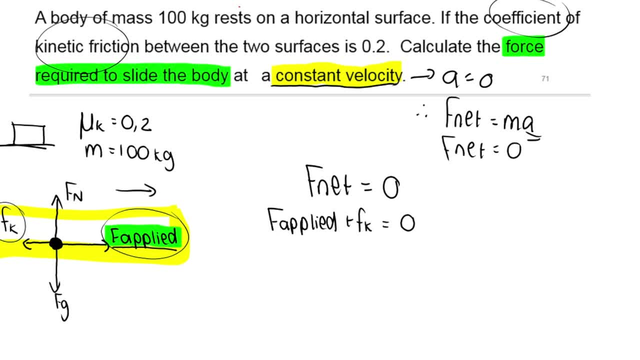 why? because the box is sliding, so the sum of these forces adding them together must give me zero. why zero? because it's a newton's first law question. acceleration is zero, so f? net is zero. and my students ask me, ma'am, must i put a plus in between? because if applied and friction are going in, 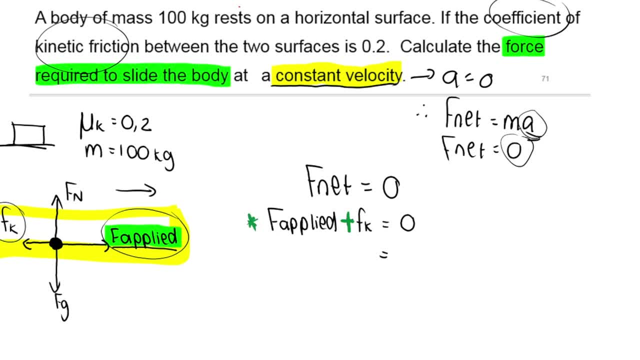 opposite directions. you always start off your equation with vector addition, which means you always start off with putting a plus sign in between when we substitute in values. that's when we'll put in a minus if necessary, and in this case it is necessary because i'm going to choose to the right. 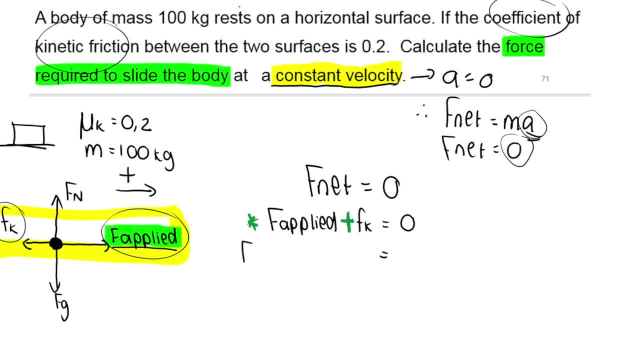 as my positive direction. so i'm looking for f applied. f applied will be going to the right. that's my positive direction. so when i substitute in a value for friction, i will substitute that in as a negative. but first i have to find friction. how do you find friction? friction, kinetic friction. 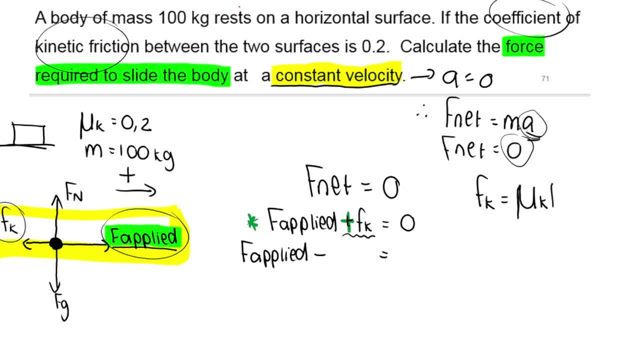 is equal to the coefficients of kinetic friction multiplied by the normal force. now, yes, they do give me the coefficient of kinetic friction. they give me that. that is zero comma two. but do they give me the normal force? no, they don't. however, i can find the normal force. look at the normal force. 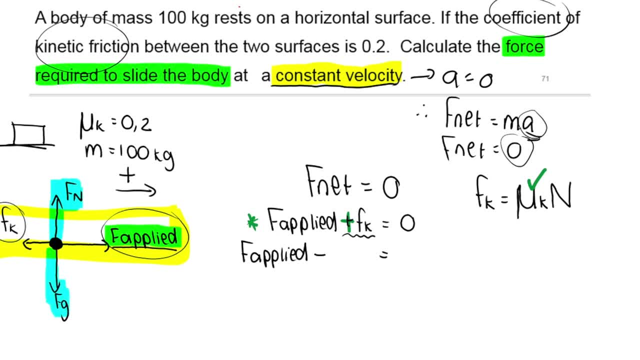 here the normal force is in the same direction as fg. there are no other forces acting perpendicularly or up or down. so what that means is, if i take those two forces, fn and fg, and i add those two together, it must also be equal to the coefficient of kinetic friction. so if i take those two forces, 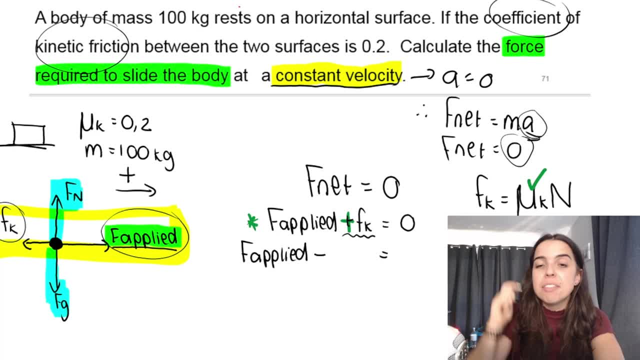 they also give me zero, which actually technically means that fn and fg have the same magnitude. think about it like this: the box is moving in this direction, not this direction. so fn and fg, those are the only two forces acting in the perpendicular direction. the box does not move. 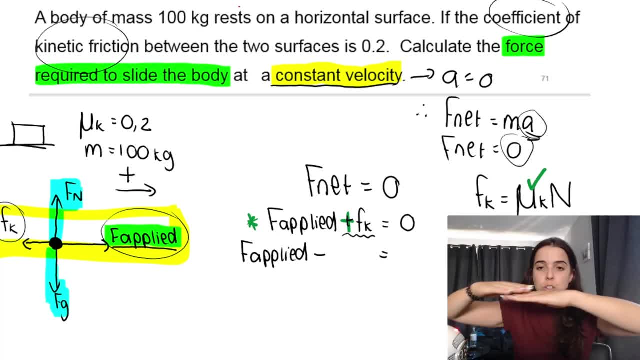 in the perpendicular direction. so it moves in the horizontal direction and it moves at a constant velocity, which means in the horizontal direction f net is zero. so if i take those two forces and i add those two forces i get zero because it's moving at a constant velocity but it's not moving at all. 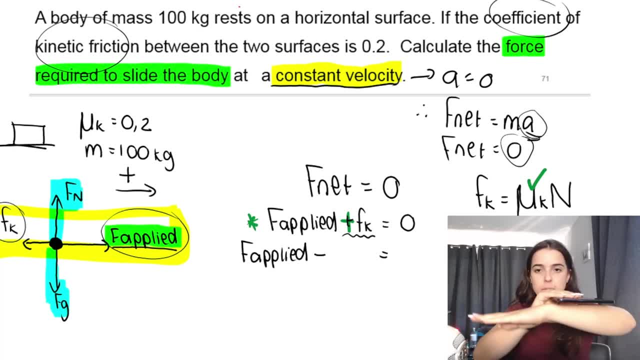 in the perpendicular direction. think about it. the box is going like this: it's not moving in the up down direction, which which means that f net in the up down direction is also equal to zero. so technically the correct way to write that in order to find the normal force is as follows: 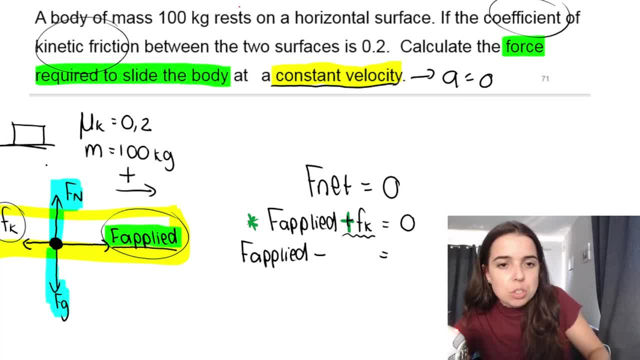 we technically should do the following: i'm going to use the two blue forces. fn plus fg must give me zero. now let's say up is positive, fn, fg is going down. do you see how it's pointing downwards? so i'm going to say minus. how do you work out fg? in the previous videos we discussed 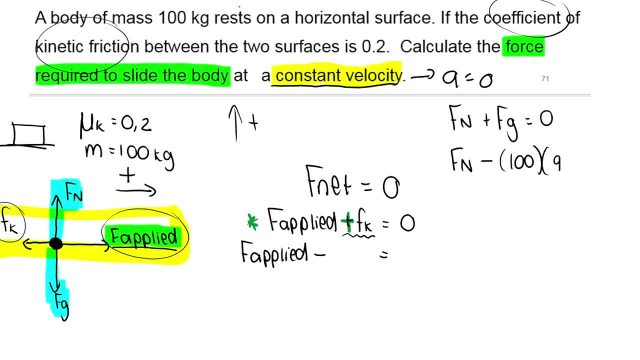 that it's mass. so 100 times gravitational acceleration 9.8, that must equal zero. so take it over fn equals, then it becomes a positive 100 times 9.8 and it will be 980 newtons upwards. and i know what you're thinking. i know what you're thinking. 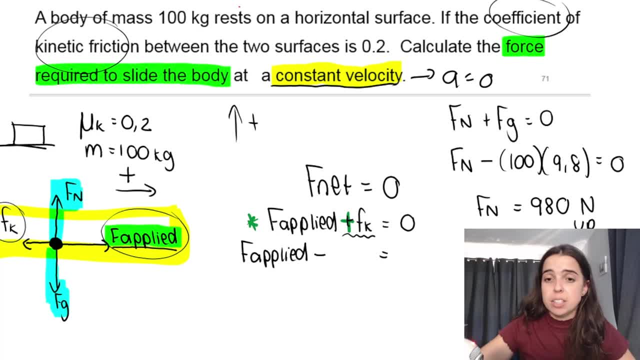 grade 11s and grade 12s. ma'am, that equation is so unnecessary because the box is on a flat surface. so that means that fg, which is 100 times 9.8, is the same as the normal force. so why can't i just 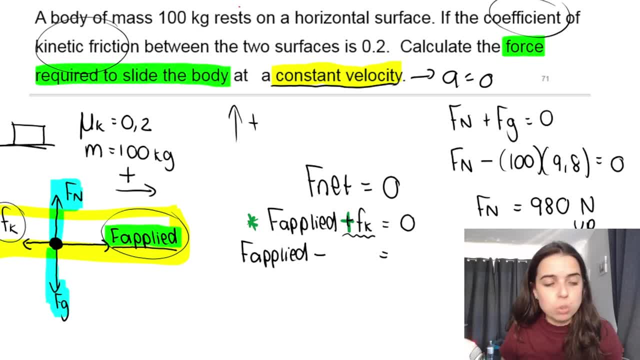 say 100 times 9.8, get the answer, and that's my normal force. you can, that is true, but remember, this is a simple example. you may get an example where fn and fg are not the only two forces acting up or down, and then you have to. 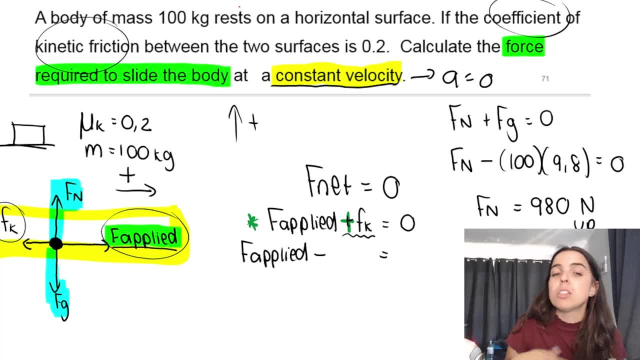 do it like this. so i want you to practice doing it like this so that when the more difficult examples come, you know what to do. okay, because if there's another vertical force acting like if applied perpendicular or something you can't say, fn is equal to fg. because it's not okay. so 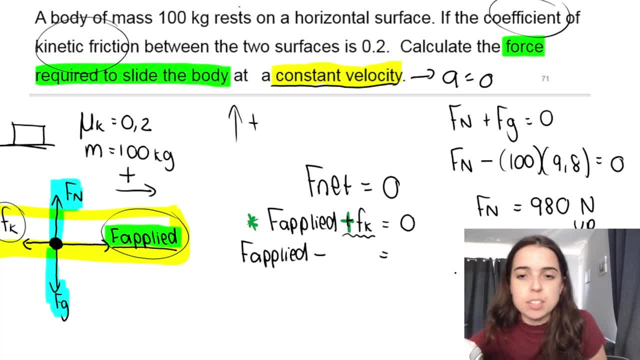 we found the normal force, which is 980 newtons up. and remember why did i want to find the normal force? well, because it's not the normal force, it's the normal force. it's the normal force because i was looking for fk. remember fk- frictional force, is equal to the coefficient of kinetic.